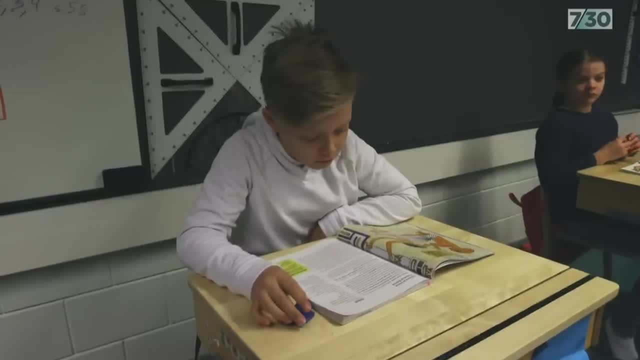 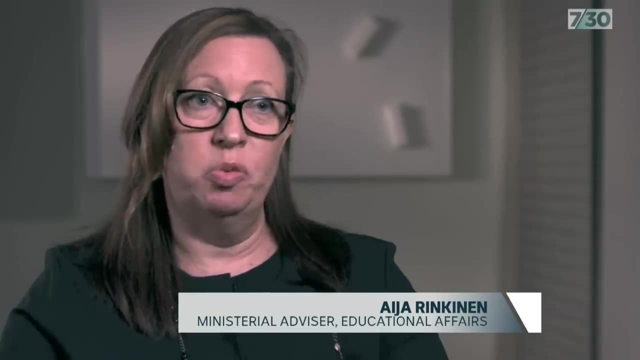 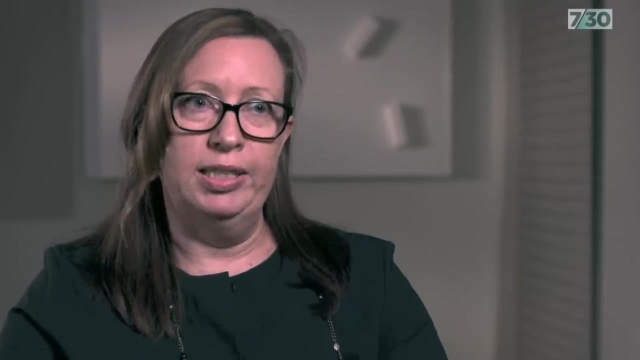 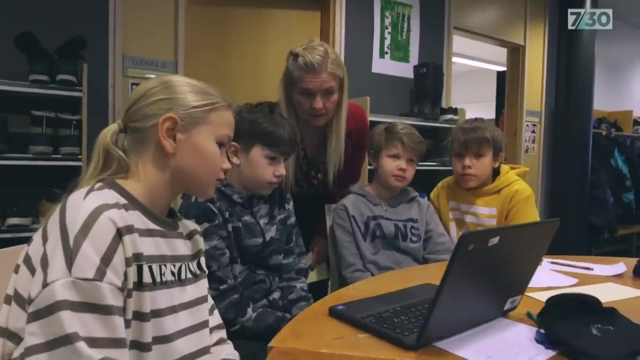 half as much time in a classroom as Australian children. When you go to the first grade, when you are seven years old, the amount of hours is 20 hours a week. It's the minimum And then it gets more hours the older you get, but it's still less than in many countries in Europe or in the world. 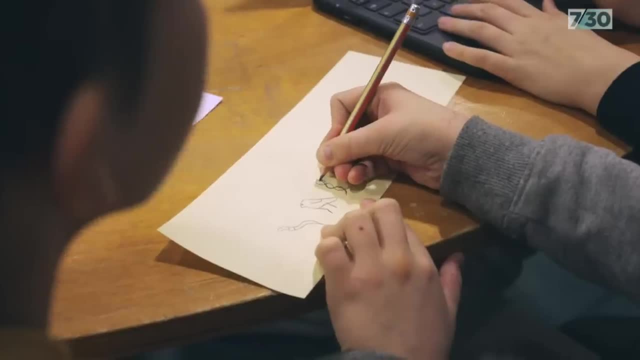 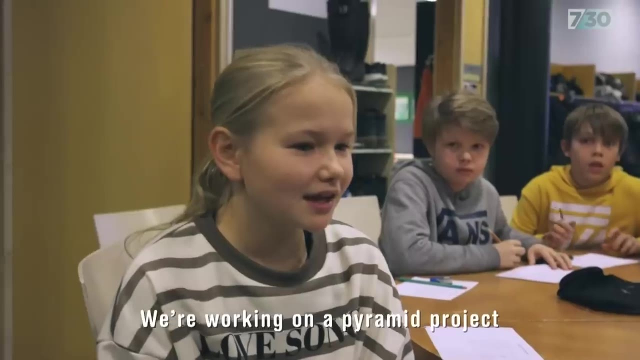 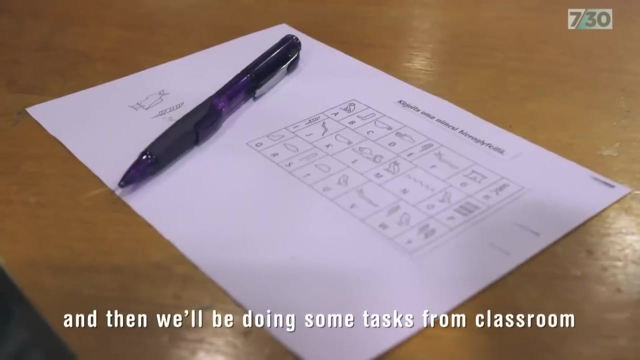 In Finland, it's individual teachers who decide how the curriculum is taught, including how much technology should feature in their classrooms. We make pyramids, We make pyramids, We make pyramids. We have a yoga and ligha project where, for example, we now funny- we write our names. 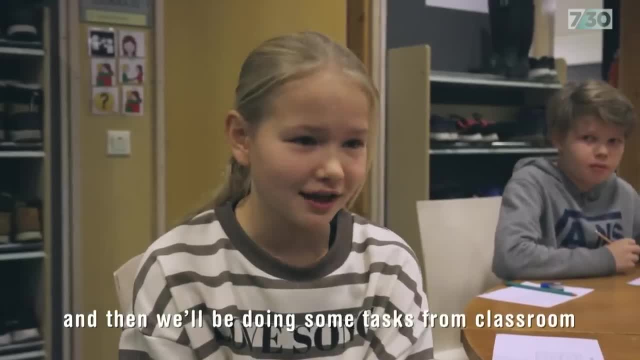 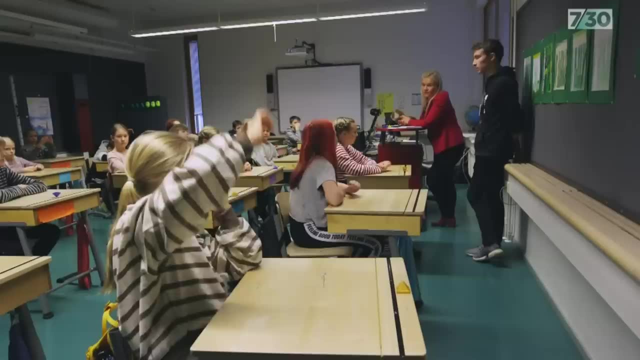 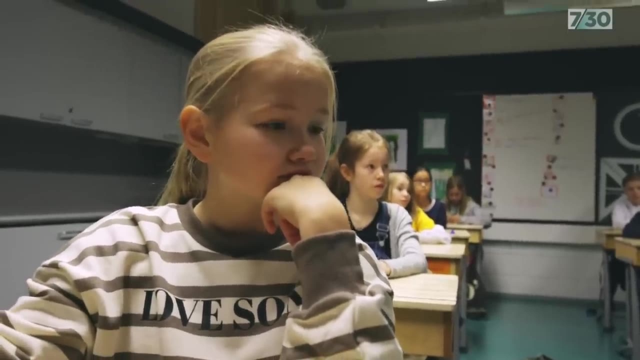 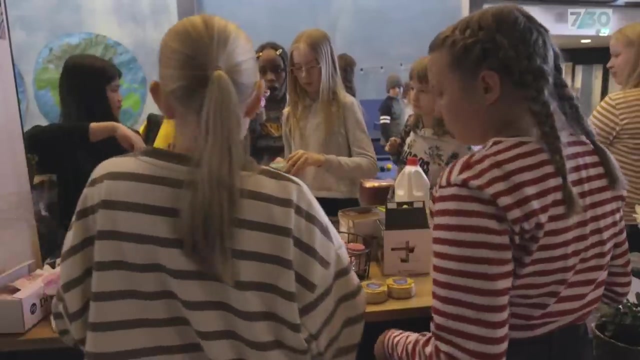 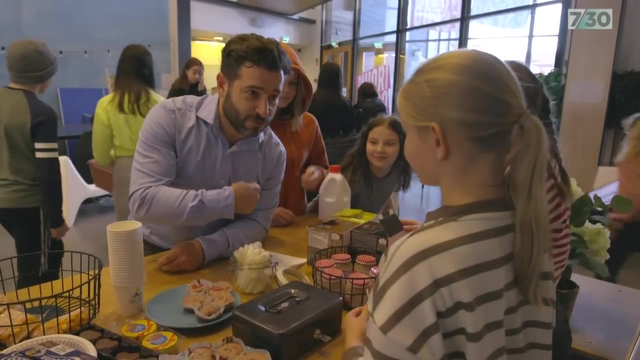 on papier posters and then we make classes from classrooms. Eleven-year-old Mintu Latomaki asks to leave class to work at the school's own student-run cafe. You can go. Yeah, that's okay, Sorry, Hello. One cake for the cameraman, one cake for me and two coffees. 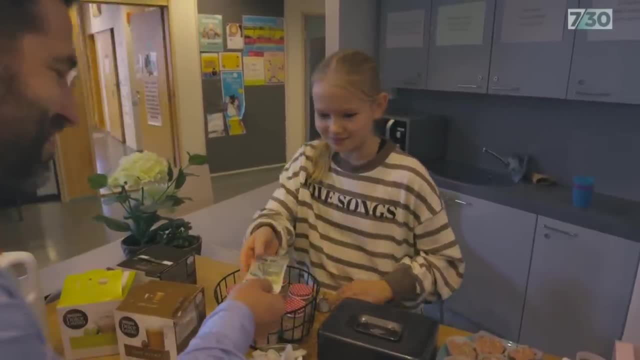 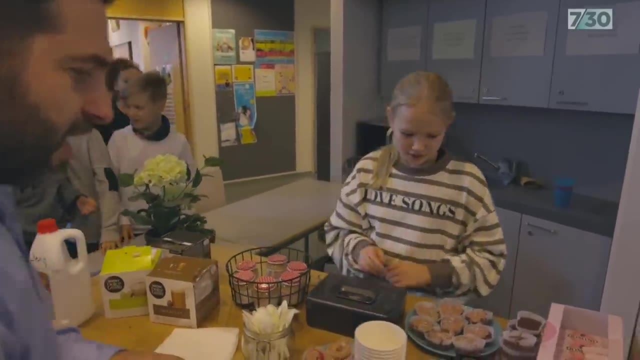 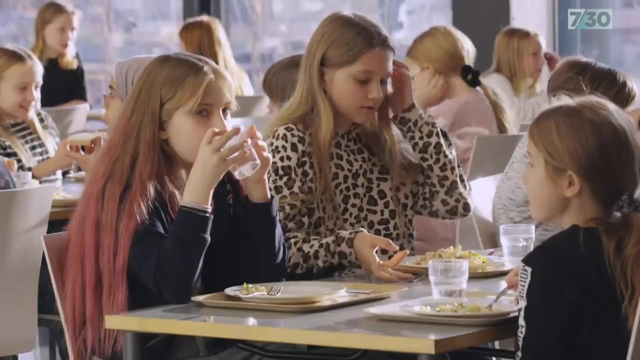 How much is it? €2.60.. How much change? €2.40.. Ketos, Perfect. Is there a tip jar? Do you have tips? No, No tips. Okay, In Finland, school lunches, like books and excursions, are free. 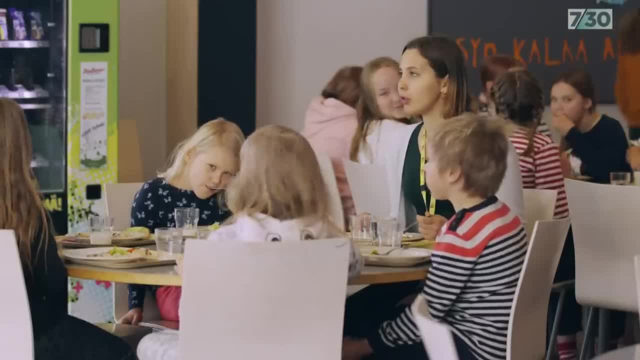 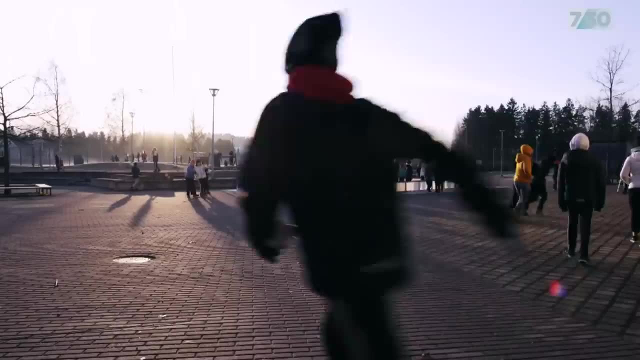 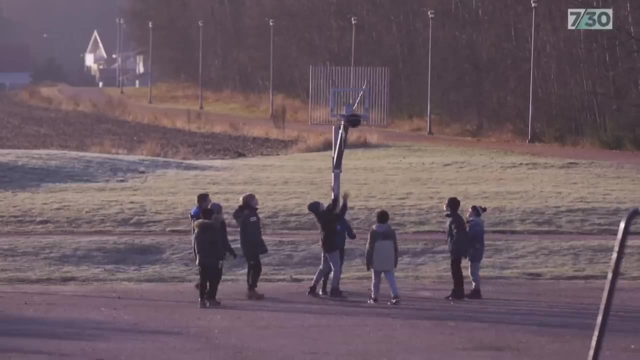 The kids select what they want, sit down with their friends and teachers to eat before they clean up after themselves. The children rug up again to play outside. Some play a raucous version of soccer, some play basketball, while others wait for the. 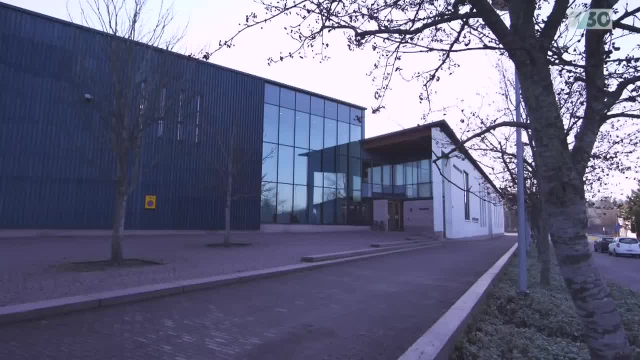 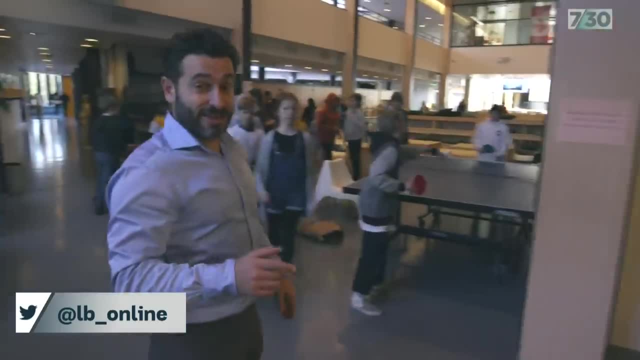 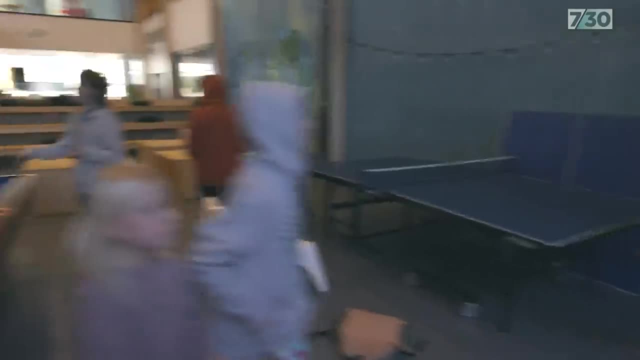 hockey rink to open. There are plenty of options for bad weather days too. The facilities, The facilities in this school are just amazing. Outside we saw an ice skating rink, and in here, where the kids can play, at lunchtime there's a ping pong table, a pool table, and in here for the cold winter days they've 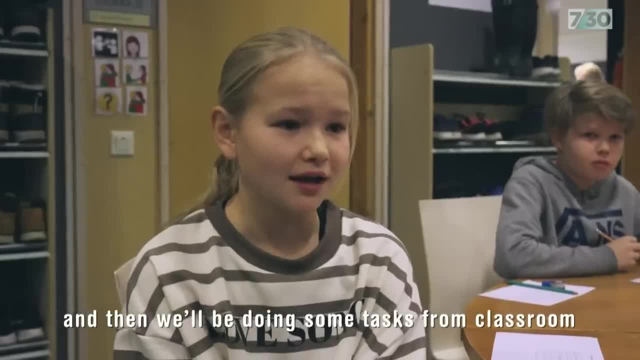 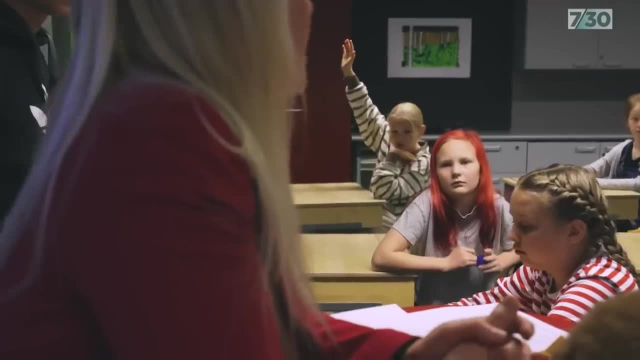 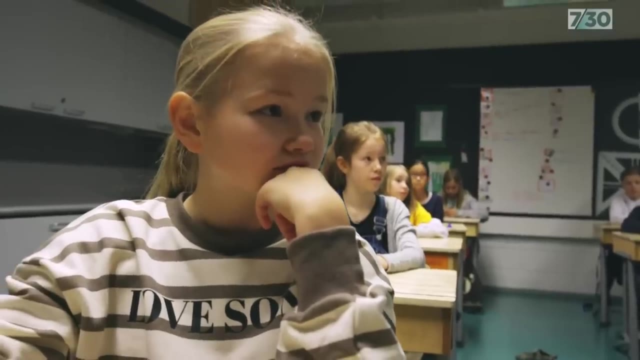 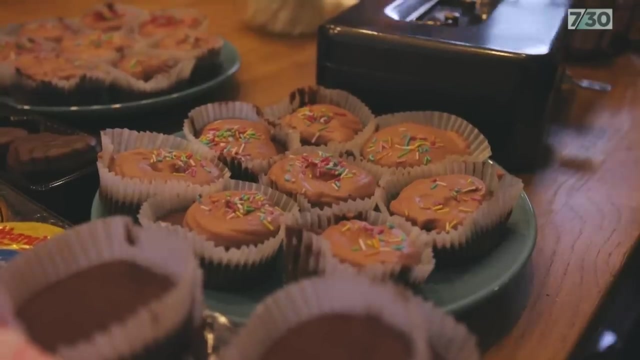 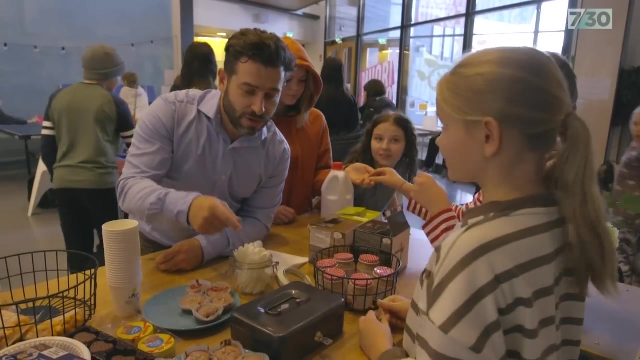 example at my hero glyphs, and then we do projects from the classroom. Eleven-year-old Mintu Latomaki asks to leave class to work at the school's own student-run cafe. You can go. Yes, that's okay. Hello, One cake for the cameraman, one cake for me and two coffees. 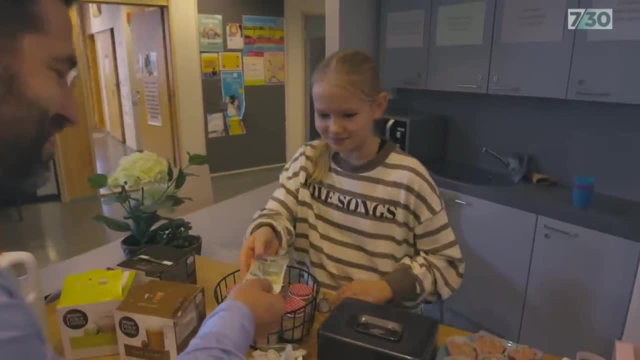 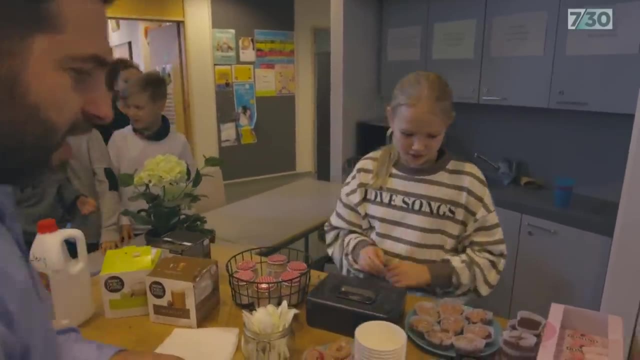 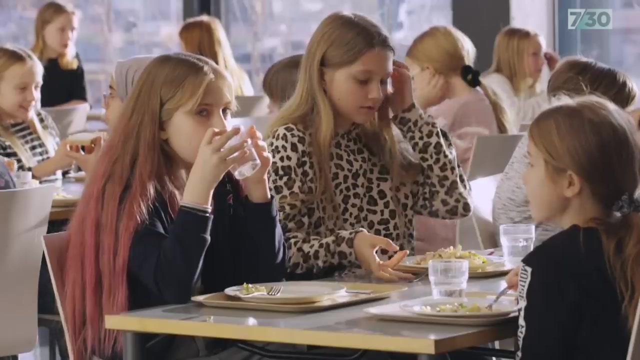 How much is it? Two euros and sixty cents? How much change? Two euros and forty cents? Ketos, Ketos, Perfect. Is there a tip jar? Do you have tips? No, No tips. okay. In Finland, school lunches, like books, and excursions, are free. 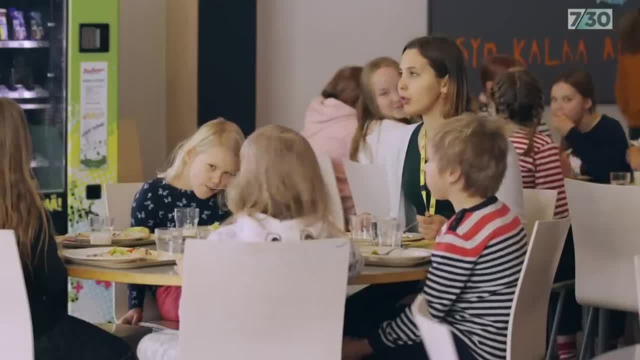 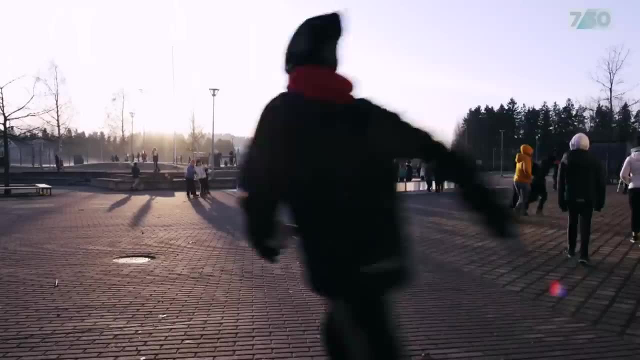 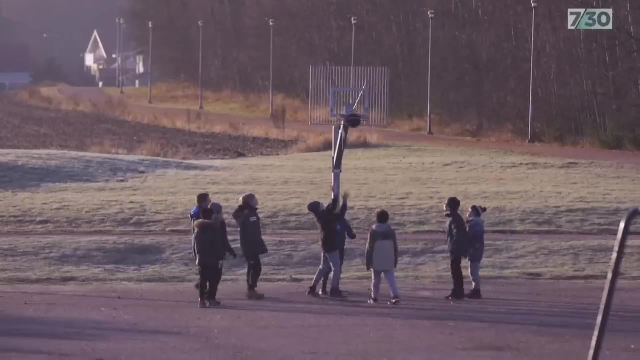 The kids select what they want, sit down with their friends and teachers to eat before they clean up after themselves. The children rug up again to play outside. Some play a raucous version of soccer, some play basketball, while others wait for the. 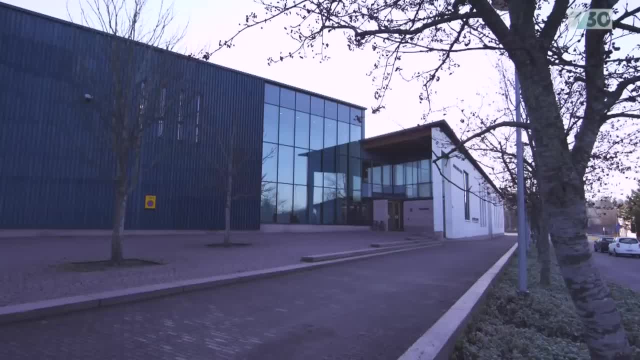 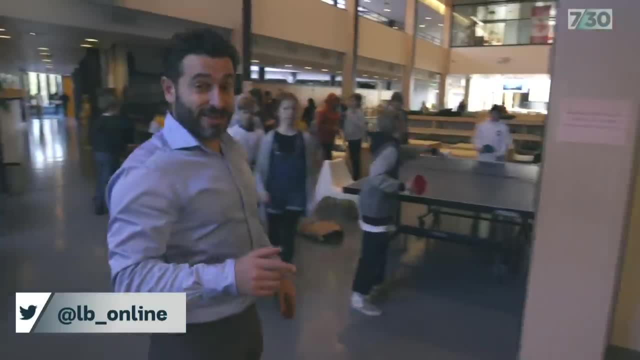 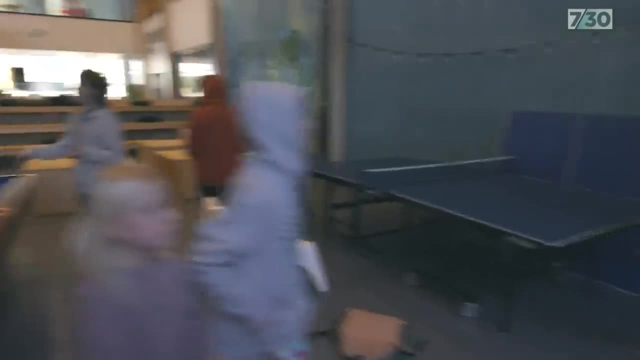 hockey rink to open. There are plenty of options for bad boys, Bad weather days too. The facilities in this school are just amazing. Outside we saw an ice skating rink, and in here where the kids can play. at lunchtime there's a ping pong table, a pool table, and in here for the cold winter days they've got. 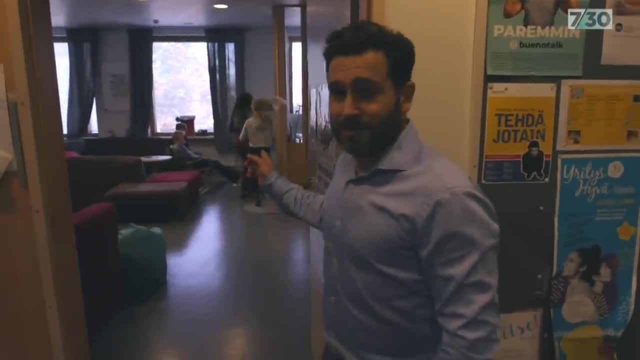 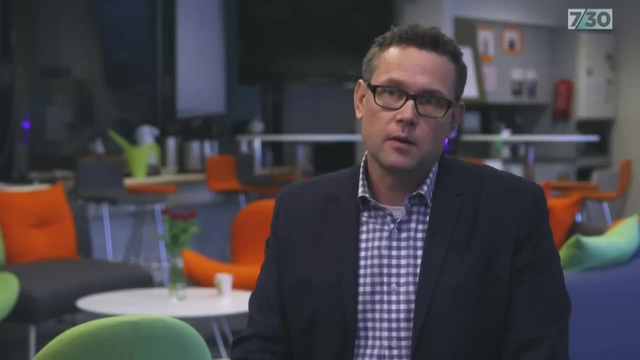 a room full of bean bags and couches, and there's even a PlayStation in the corner. It seems like it's such a rich school you must get more money than other schools. No, we don't. It saves money for everyone actually. 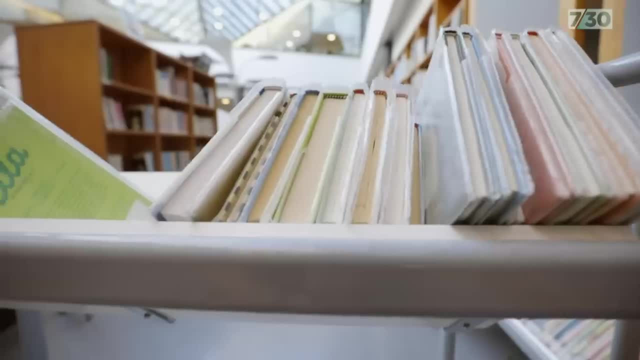 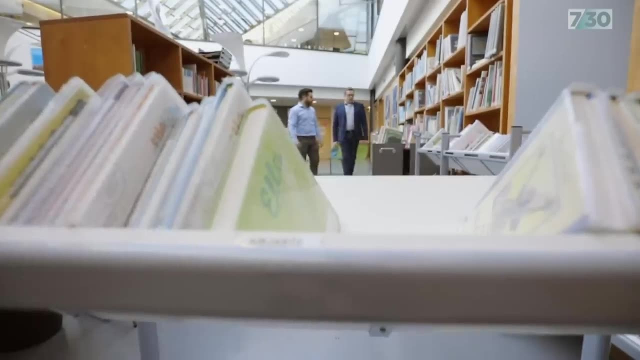 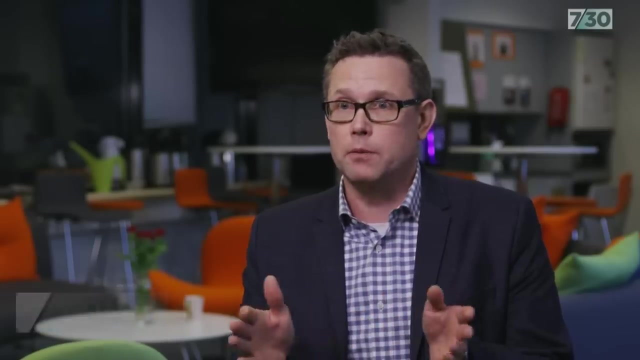 They take and borrow books. In Finland, schools are not allowed to raise private funds or to charge fees from parents. All schools are equitably funded from taxation And in our system everything is free for the students. actually, We don't collect any money from the parents. 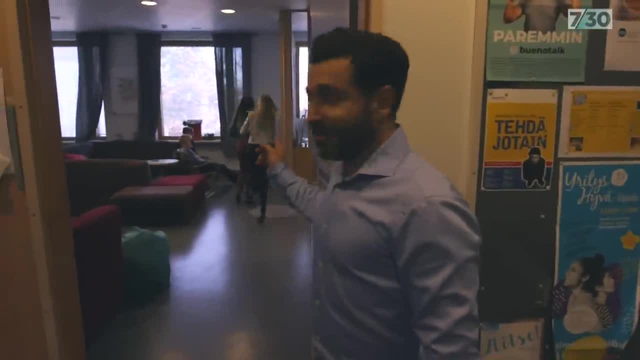 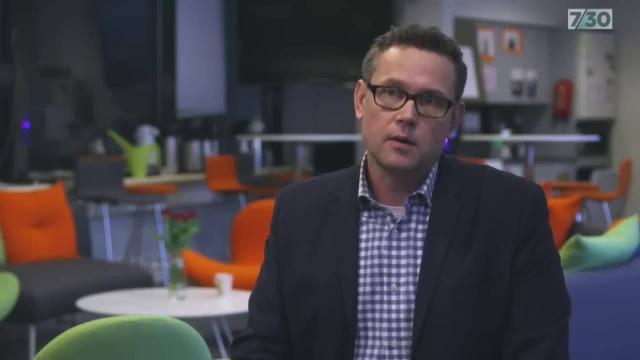 got a room full of bean bags and couches and there's even a PlayStation in the corner. It seems like it's such a rich school you must get more money than other schools. No, we don't. It saves money for everyone actually. 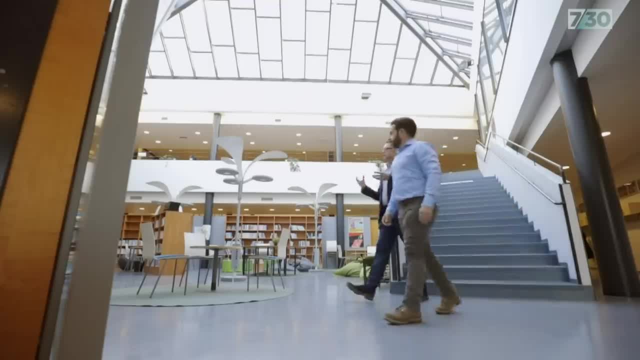 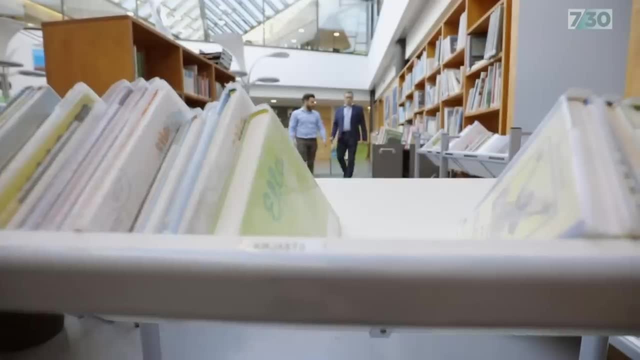 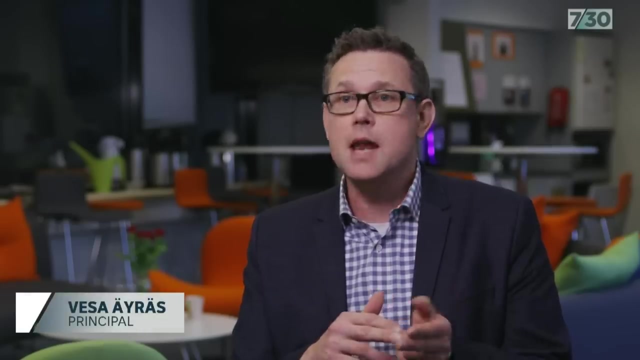 They take and borrow books. In Finland, schools are not allowed to raise private funds or to charge fees from parents. All schools are equitably funded from taxation And in our system everything is free for the students. actually, We don't collect any money from the parents. 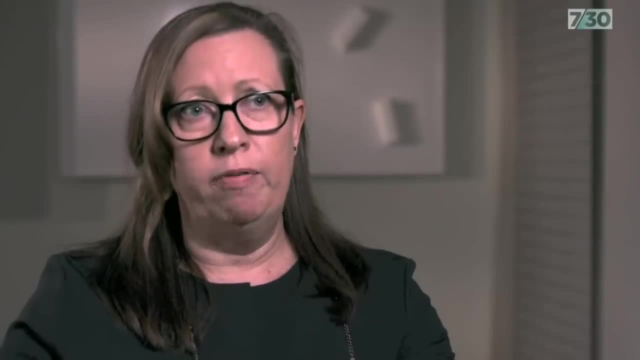 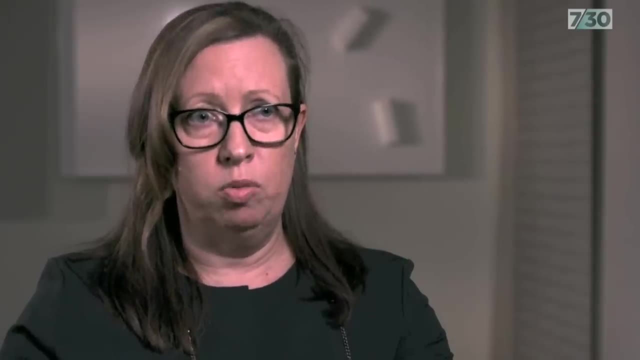 We want our schools to be equal and have the equal opportunities to arrange the education. So therefore also the finance system needs to be equal. So therefore also the finance system needs to be equal. So therefore also the finance system needs to be equal. 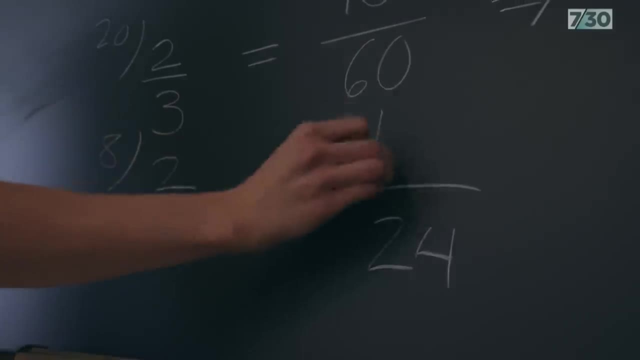 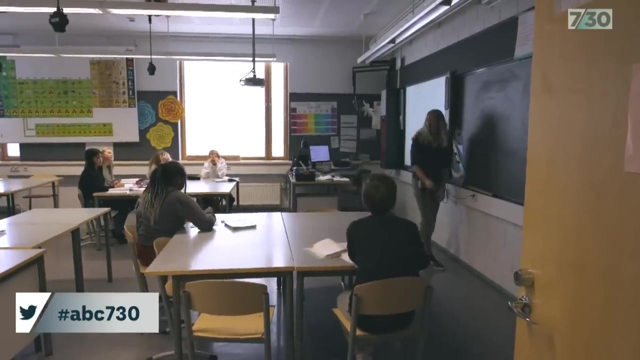 And treat equally all the schools. And then here we have 16.. Minto Latomaki's older brother, Levi, is in year 7, and this afternoon he's got maths. Minto Latomaki's older brother, Levi, is in year 7, and this afternoon he's got maths. 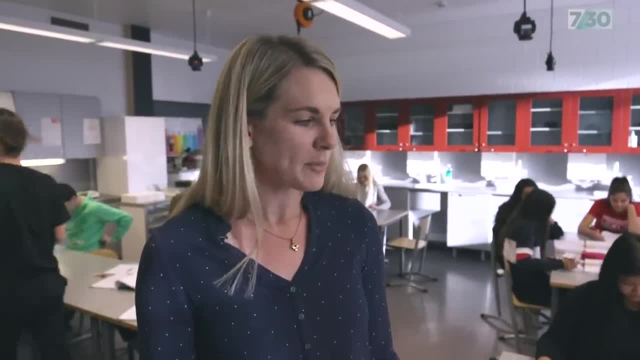 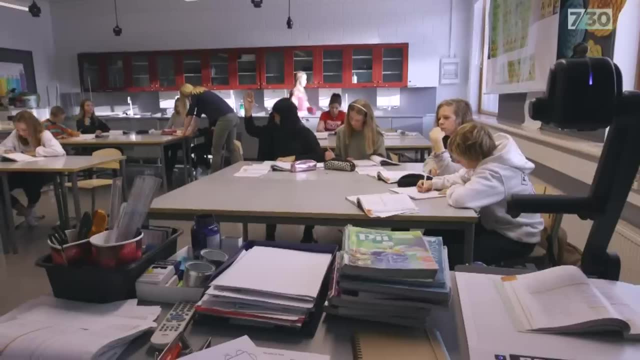 We have the last chapter before we have the next exam. There are regular exams in Finland, but the results of these tests are not published and shared. We have national tests, but the big difference is in the number of students. We have national tests, but the big difference is in the number of students. 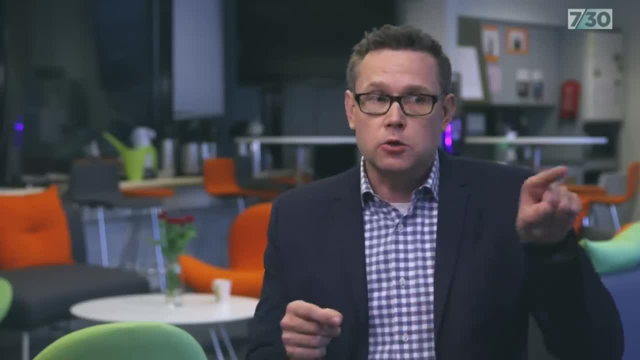 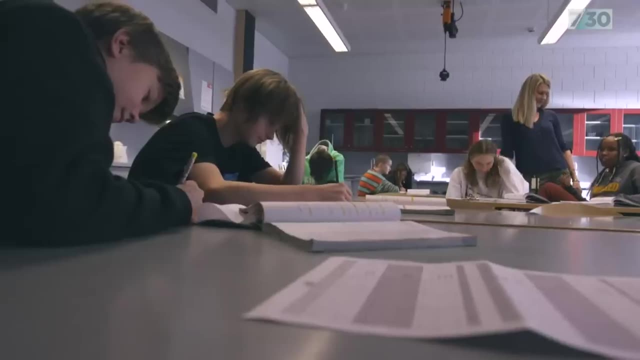 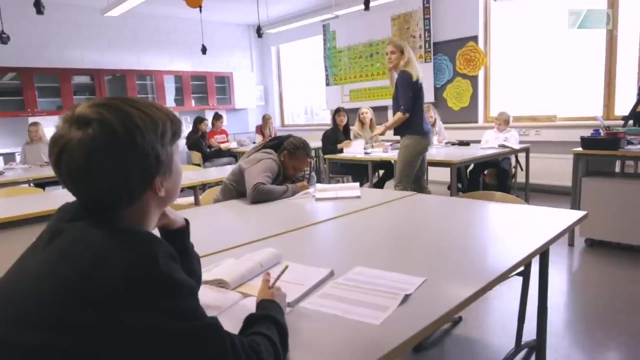 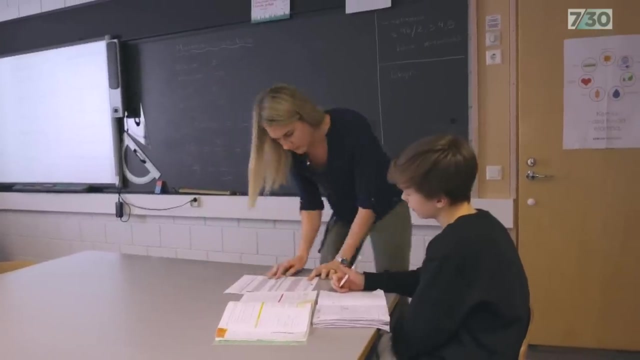 differences. we don't compare schools, that this is not good school, this this is bad school, and we just used information that we evaluate ourselves. but perhaps the single biggest difference in Finnish education is the standard of teaching. Levi's maths teacher, Una Arnes, speaks five languages and has postgraduate qualifications. so every one of us, we have to have a. 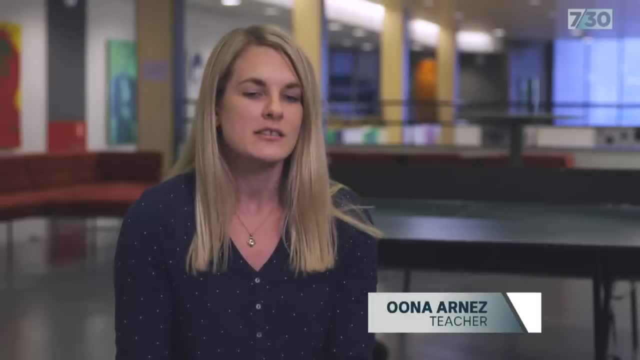 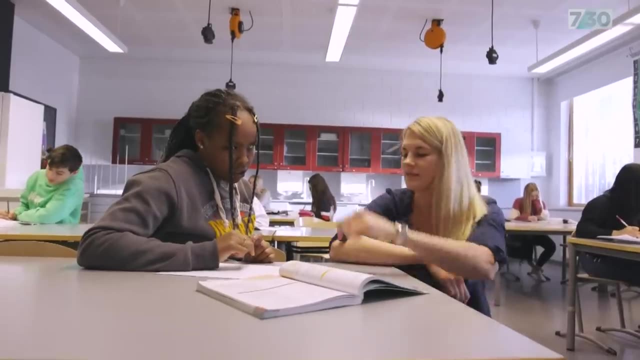 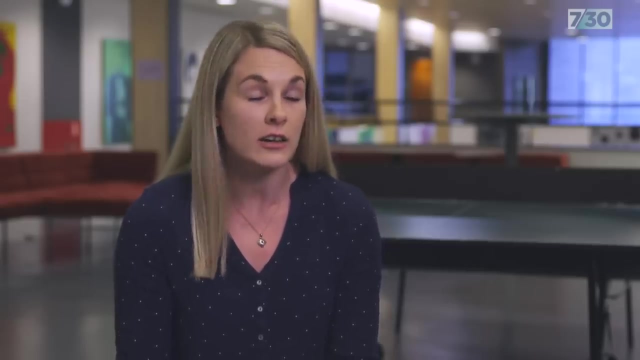 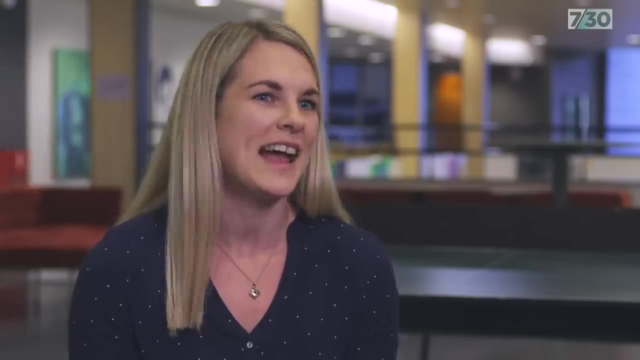 master's degree to to be teachers. so, like, for example, me, I'm math and chemistry and physics teacher. in Finland, a career as a teacher is highly sought after. to enter the studies in university actually it's really hard. they take something like 10% to study teaching. if you really want to be a teacher, it can't. 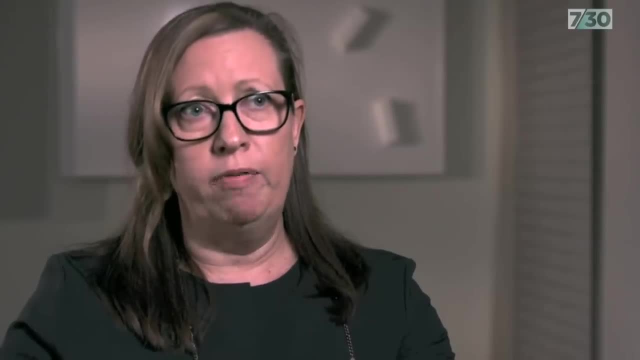 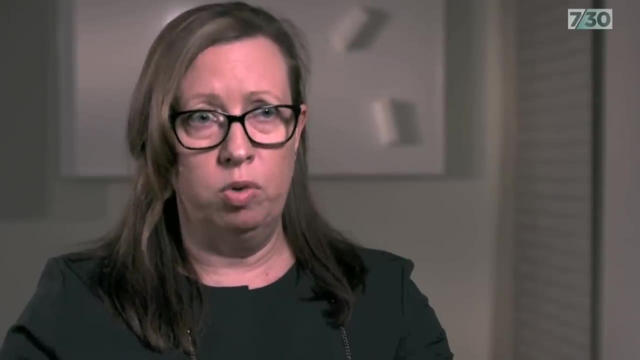 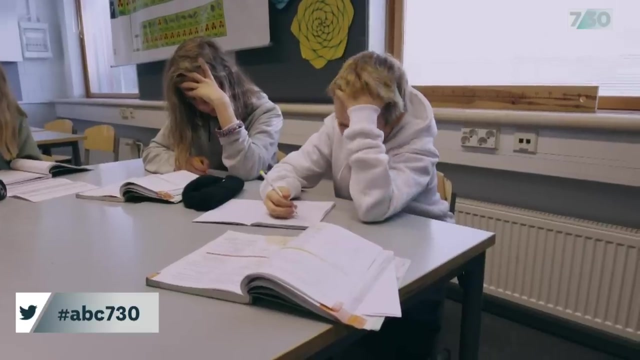 We want our schools to be equal and have the equal opportunities to arrange the education. So therefore also the finance system needs to be equal and treat equally all the schools, And then we get 16.. Mintu Latomaki's older brother, Levi, is in year seven and this afternoon he's got maths. 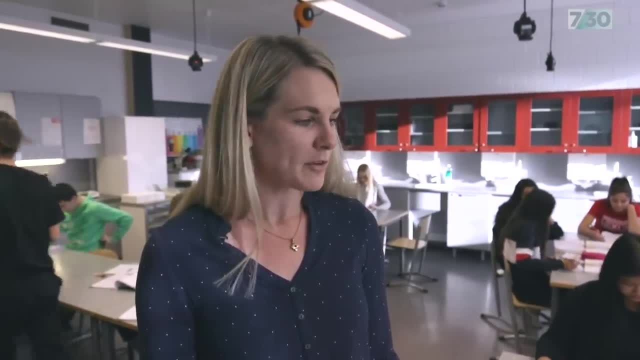 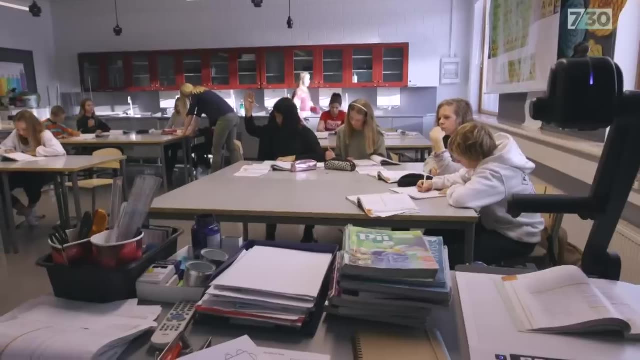 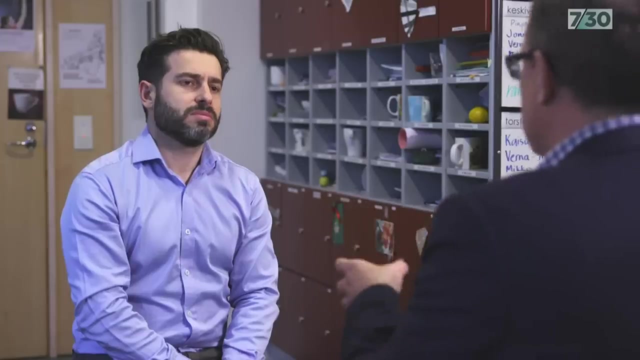 We have like the last chapter before we have the next exam. There are regular exams in Finland, but the results of these tests are not published and shared. We have our tests, but the big difference is we don't compare schools. that this is not a good school, this is a bad school. 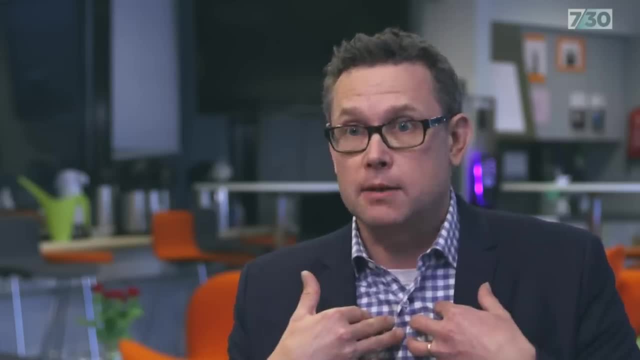 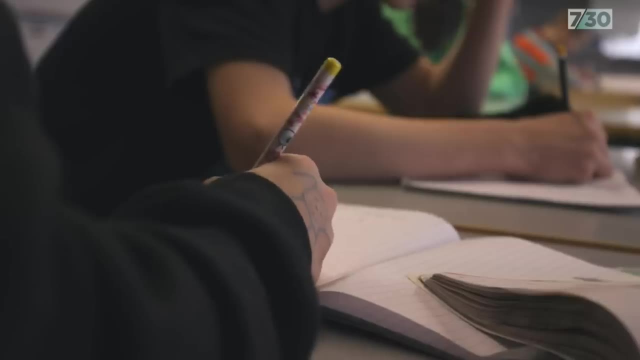 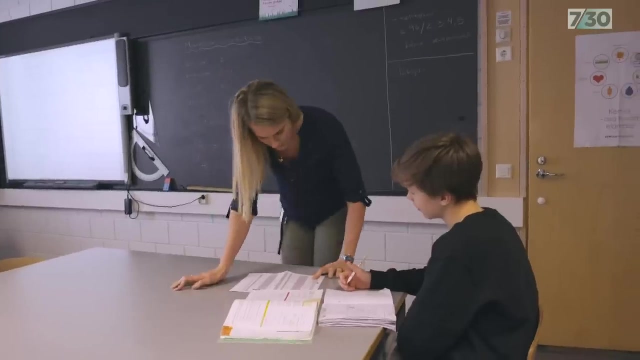 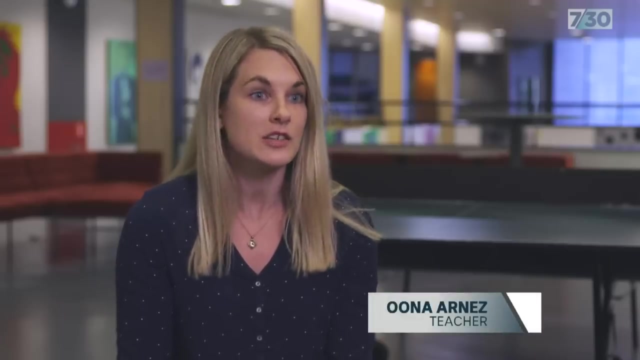 We just use the information that we evaluate ourselves. But perhaps the single biggest difference in Finnish education is the standard of teaching. Levi's maths teacher, Una Ahnes, speaks five languages and has postgraduate qualifications. So every one of us- We have to have a master's degree to be teachers. 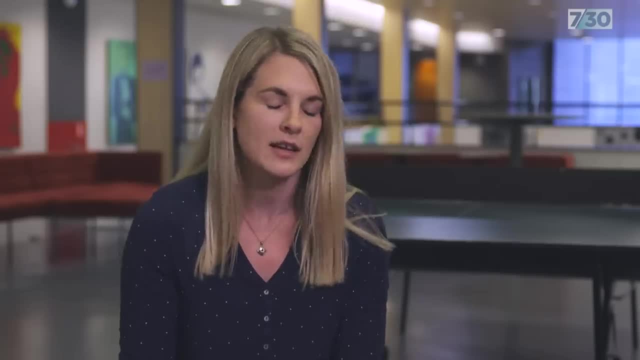 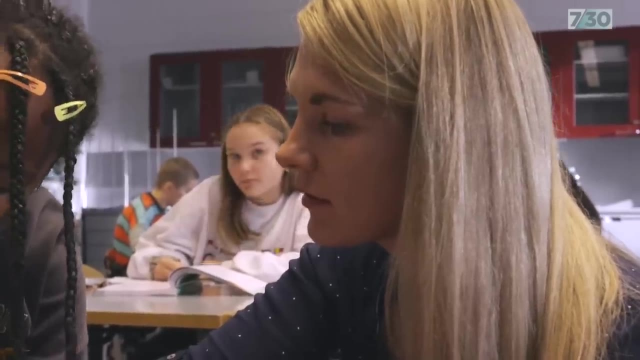 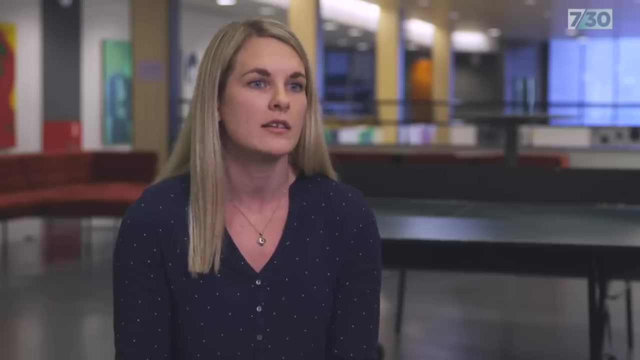 So, like, for example, me, I'm a math and chemistry and physics teacher. In Finland, a career as a teacher is highly sought after. To enter the studies in university actually it's really hard. They take something like 10% to study teaching. If you really want to be a teacher, it can't be your second or third or I don't know what. 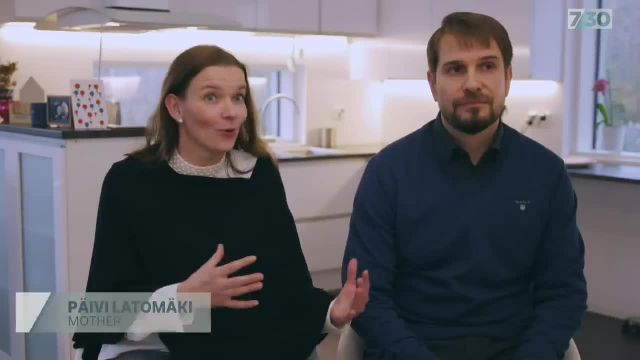 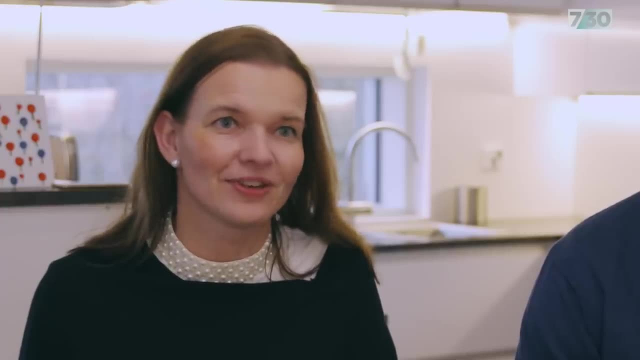 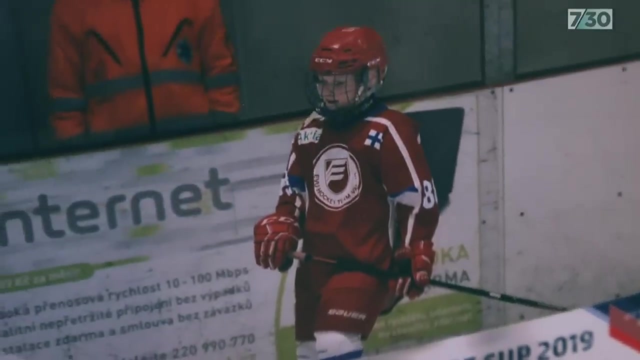 kind of option. It has to be your first. I believe that they know what is the best for our children. I'm not a teacher, I don't have that education, So we don't interfere their work. In Finland there's little anxiety about finding the right school for your child. 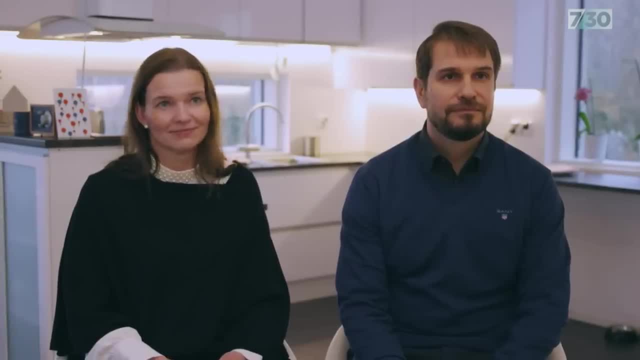 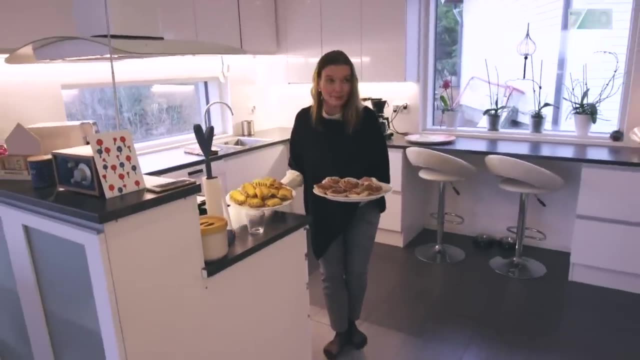 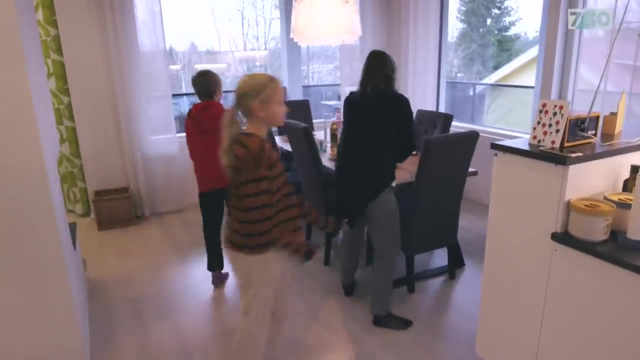 We trust that they have a very good school, so we don't need to do any research work. I think that is not a question in Finland. No, no, No, No, No. We are a very different country, with a tiny, homogeneous society, but its education success. 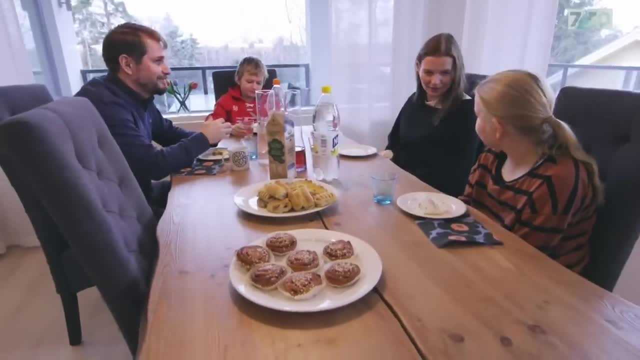 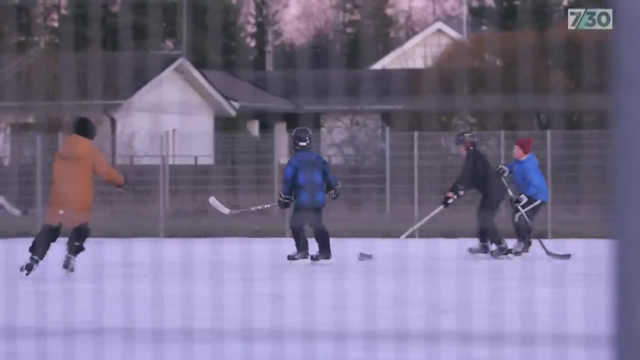 must surely offer some lessons for Australia. I would like to say that try to build the system that you trust the people And its investment in teachers seems an obvious place to begin. The society respects the teachers. it means also the parents respect the teachers and